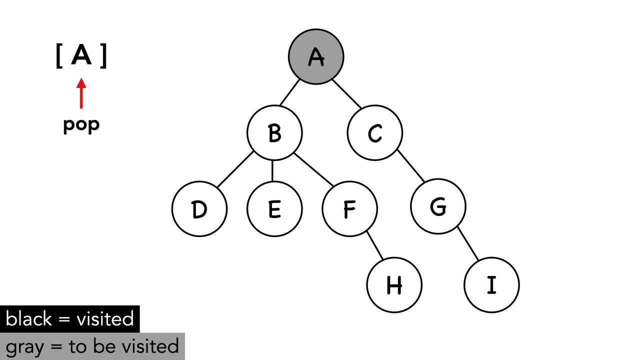 corner. We pop A from the queue and mark it as visited. We also add its adjacent nodes into the queue. B is the next node out of the queue. We mark it as visited and add its adjacent nodes into the queue. Same with C. 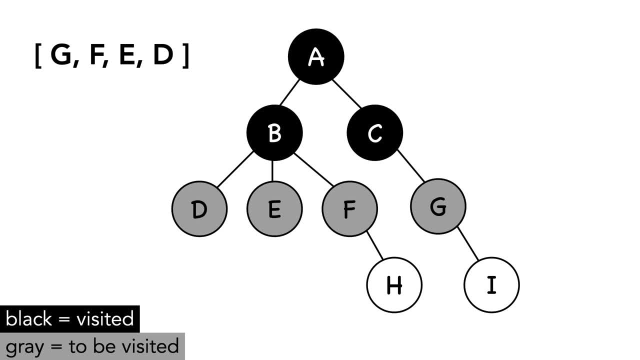 Here I'll pause our algorithm and illustrate what we mean by breath. We visit nodes at the same level before we progress vertically. D is the next node out of the queue that are in line to be visited. We mark it as visited and add its adjacent nodes into the queue. 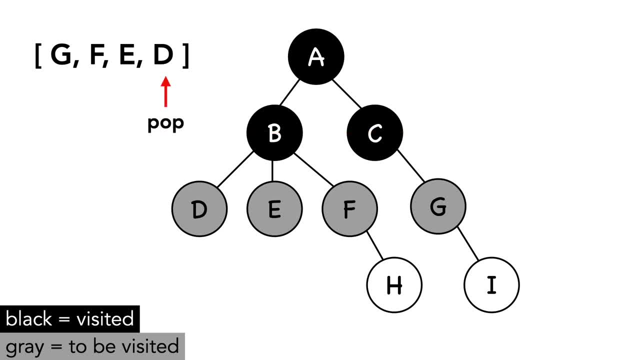 B is the next item out of the queue. that are in line to be visited. that are in line to be visited. I'll let the rest of the algorithm finish. without voiceover stabilizer, There is nothing left in the queue, so our algorithm is finished. 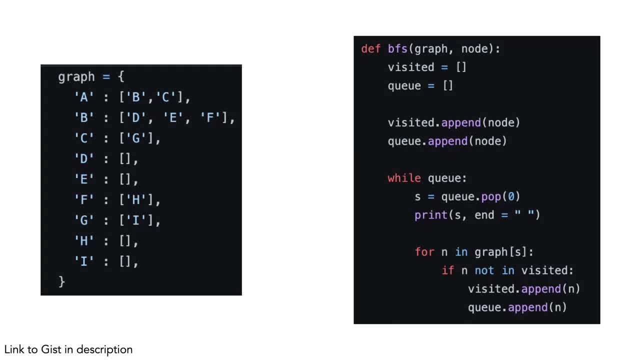 Without a word, we have reached the next node. Here is the code for Breath First Search. Without a word, we have reached the next node. out of the queue dawn to a working Python example. in the description On the left is our graph represented as an. 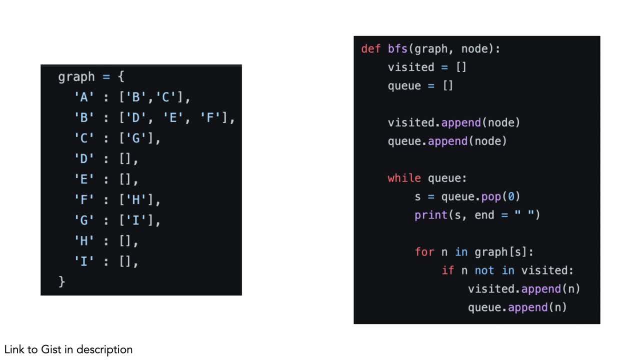 adjacency list. Let's walk through the code on the right. We first add the root node to both the visited list and the queue. We loop while the queue is not empty, removing the node that was first added to the queue. We iterate through the adjacent nodes and if the node has not yet, 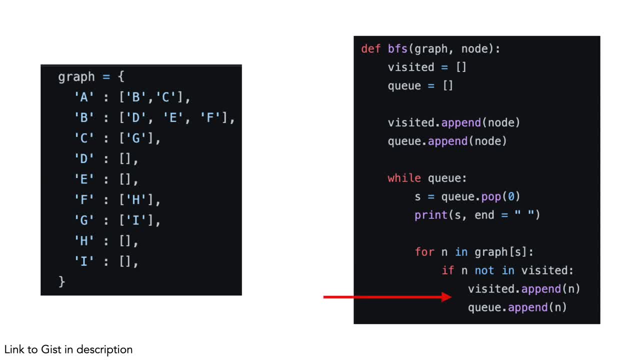 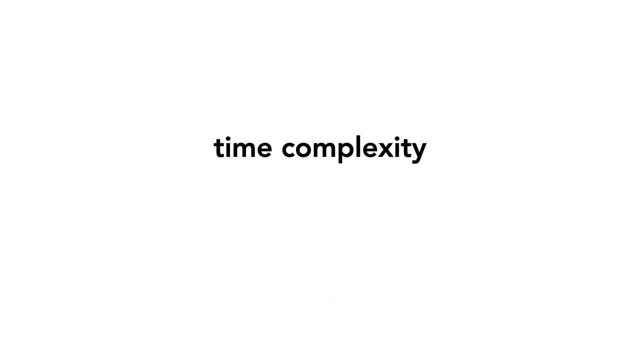 been visited, we add it both to the visited list and the queue. Let's discuss time complexity. If you think about our example, in the worst case we're going to visit each node and explore every edge. Therefore, the time complexity of BFS is big O of the number of vertices. 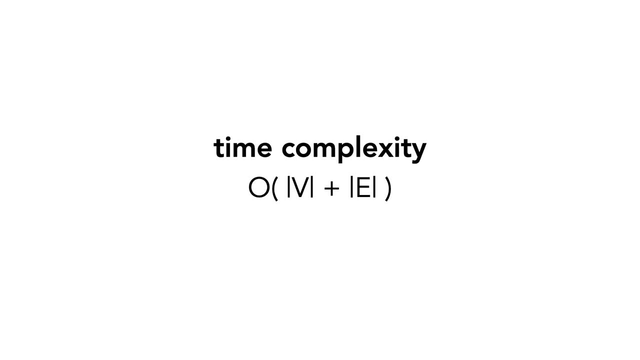 plus the number of edges. Thank you for watching. Please subscribe and share. Thank you for watching.